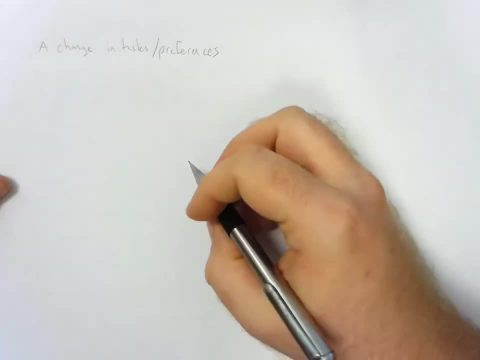 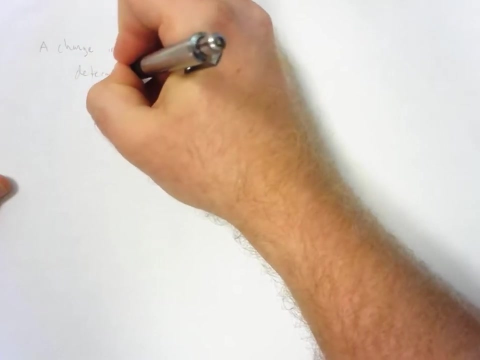 Alright, today we're going to go over how the taste and preferences, or, more specifically, a change in taste and preferences, can change the supply and demand graph. So taste and preferences is one of the determinants of demand, And what that means is that it can. 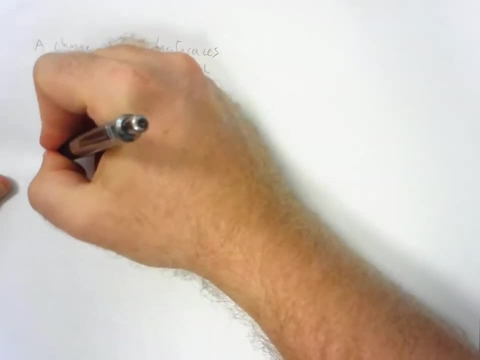 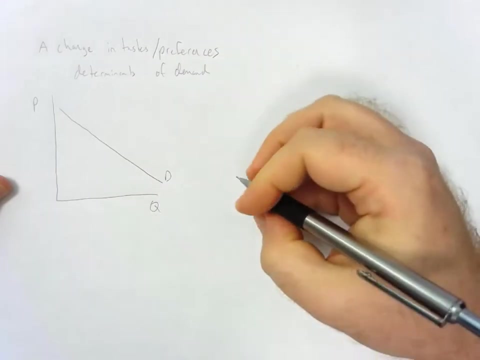 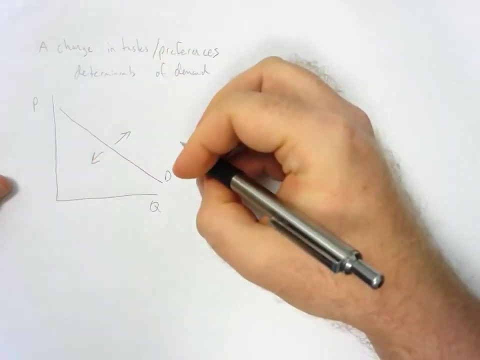 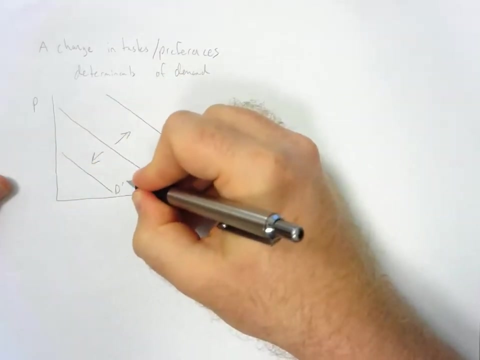 shift demand. So basically, we want to look at our classic demand curve just like that And if we see a change in taste and preferences, then we're going to see demand shift, either left or right. It could potentially increase or the demand curve could shift left, which? 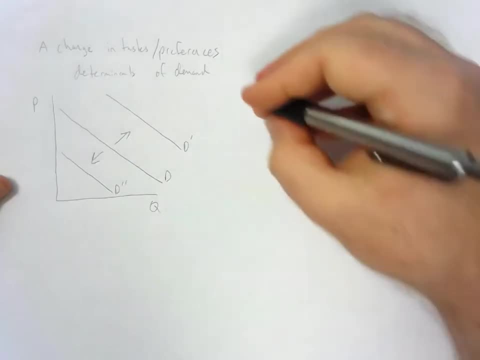 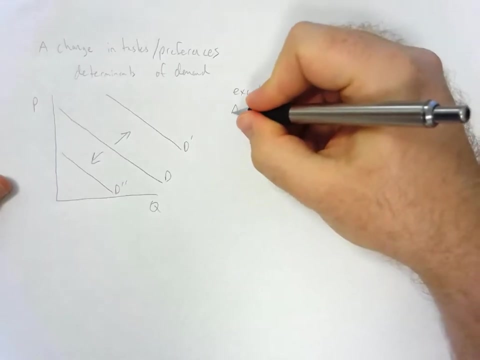 shows us a decrease in demand. So let's look at some of these, Let's look at some examples of changes in taste and preferences. So I think the classic example you could look at: apples, And maybe apples are discovered to cure cancer. 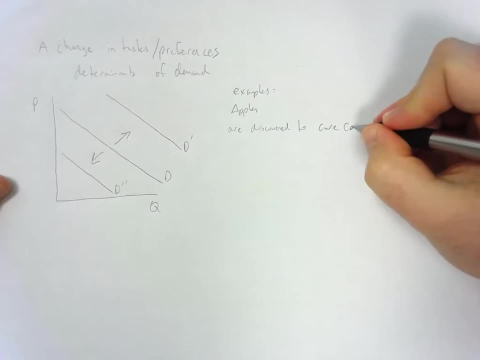 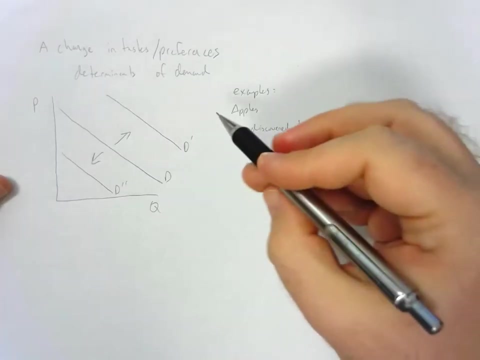 Now. granted, it may not be very realistic, but you can imagine if apples were discovered to cure cancer. that is going to definitely increase the preferences for apples, People will enjoy them a lot more and we will see an increase in demand. So what would 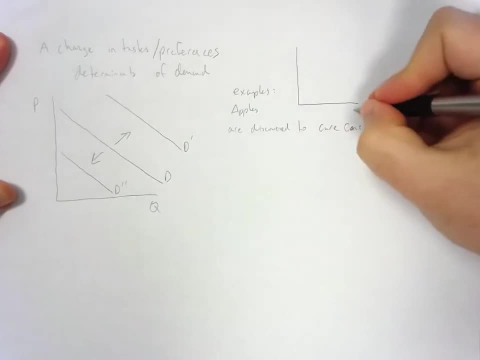 that look like in our supply and demand graph. Again, we have quantity and price, We have demand and supply. An increase in demand would cause that to shift right And you can see that this is our initial equilibrium And this is going to be our new balance. So we're. 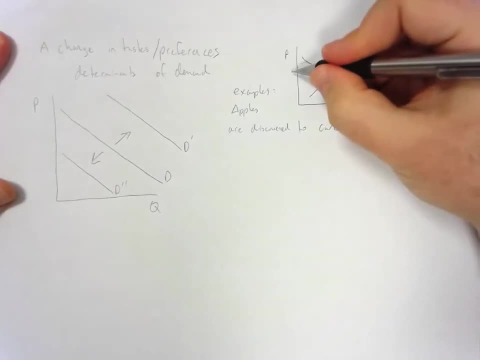 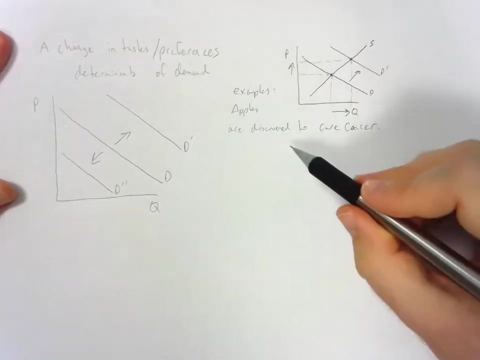 going to do equilibrium, And so what happens to equilibrium price and equilibrium quantity? They both go up. So if apples are discovered to cure cancer, as we would expect, the price is going to go way up because demand increased And equilibrium quantity will also go up. 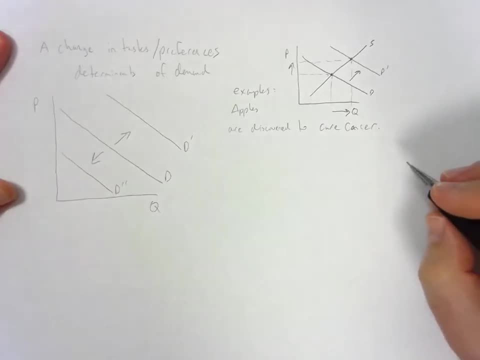 because of that increase in demand. So what's another example? Let's say LeBron James endorses Nike. Again, we would imagine the tastes and preferences for Nike products to go up. This will cause the equilibrium price to go up and the equilibrium quantity to go up.